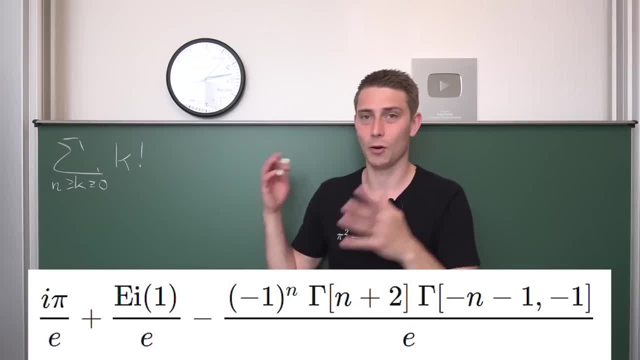 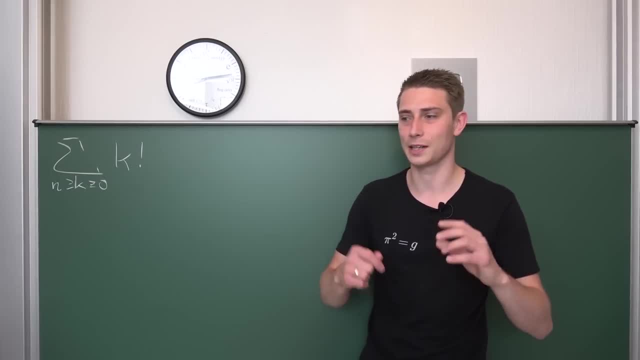 numbers, half gamma functions, So yeah, all this crazy stuff. So upper incomplete gamma functions, Blah, blah, blah. It's pretty amazing. I'm not going to derive it on this channel, though, because it would take like five to ten videos to derive this expression. Not worth it, to be honest. I would lose a lot of viewers. 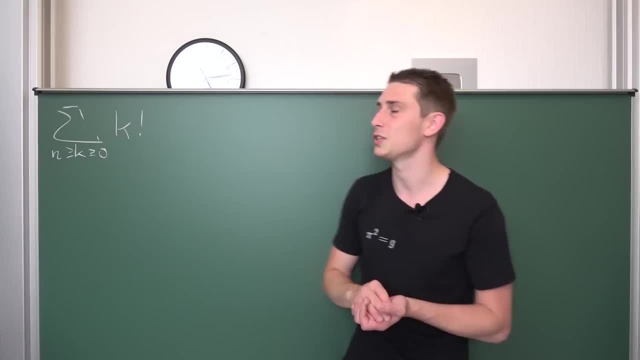 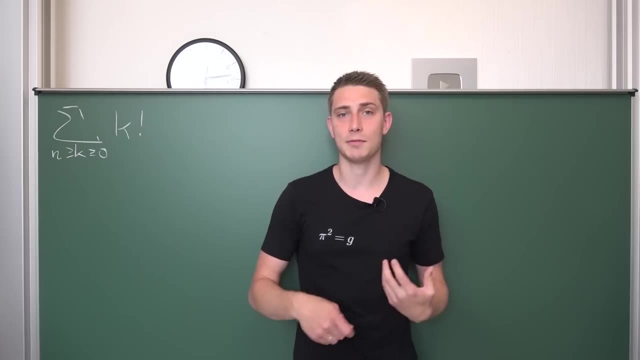 But we are going to dive right in. It's going to be kind of amazing What we are going to do today. So k factorial- We are going to extend this to an analytic continuation, and there's actually something that we are really familiar with at this point: k factorial is nothing but the gamma function of k. 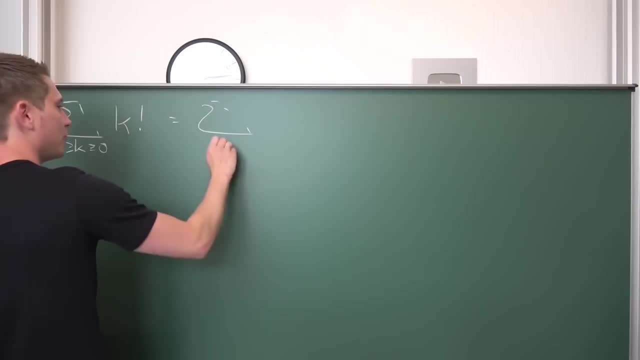 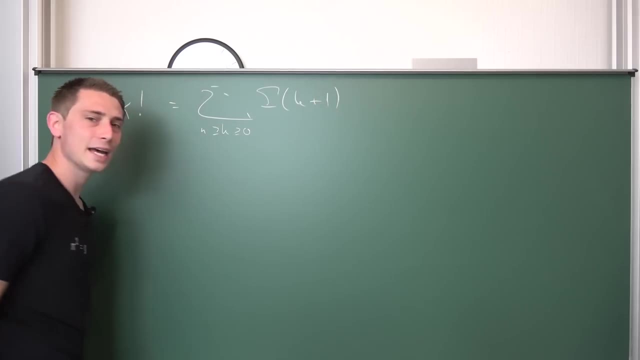 plus 1.. Okay, we are going to rewrite it. So this right here is just a finite boy, bounded between 0 and n, of the gamma function of k plus 1.. And the gamma function of k plus 1 actually allows for a nice analytic continuation to the right. 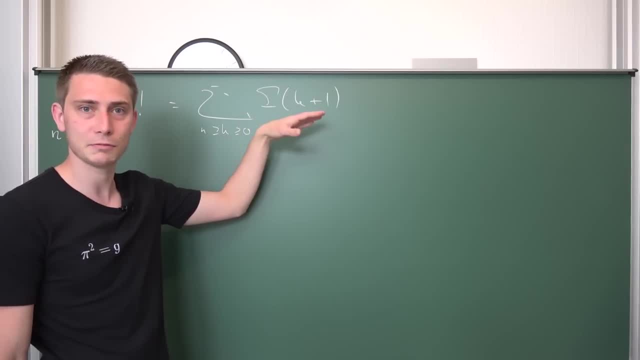 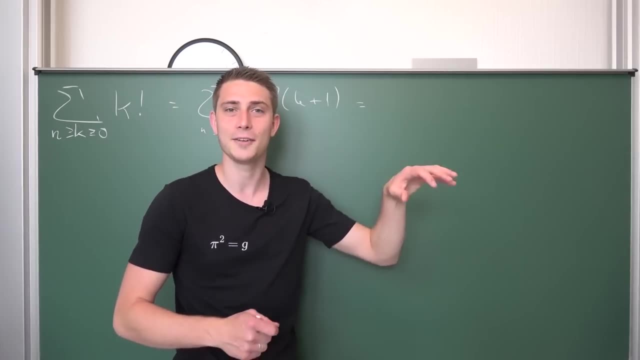 hand complex plane. That is a good thing Here, Being given by an integral representation. I have derived this thing before using Feynman integration, basically Leibniz rule for integration, and also Laplace transforms. Check it out. Link will be at the top of the. 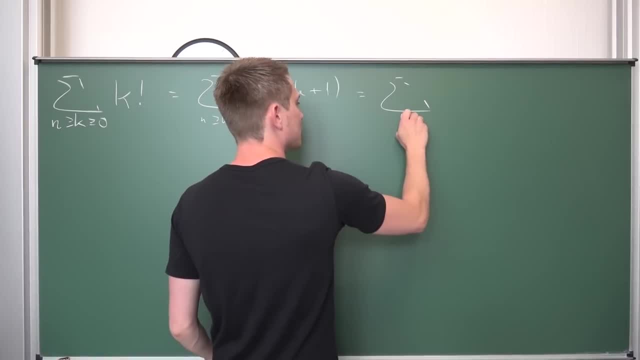 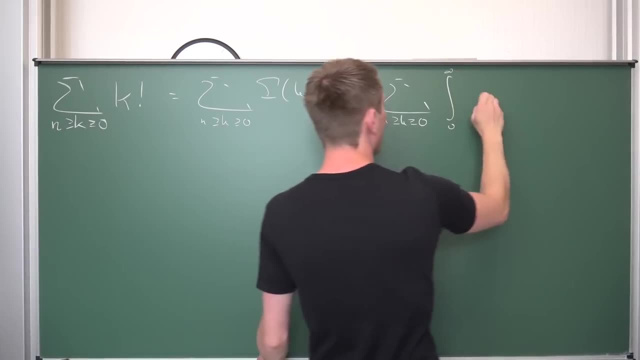 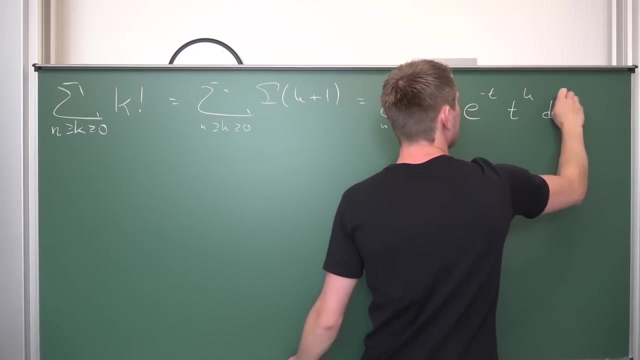 description: Pretty amazing video. So this thing right here is, on the one hand, the sum being bounded between n of the integral, from 0 to infinity, of e to the negative t. This is the variable we are integrating over Times, t to the power integrated with respect to t. and yeah, now we are halfway done already, if you see something. 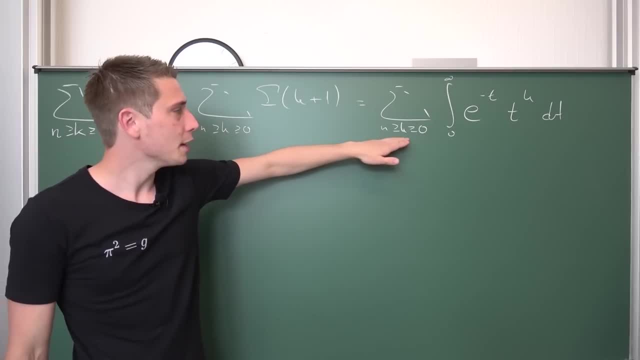 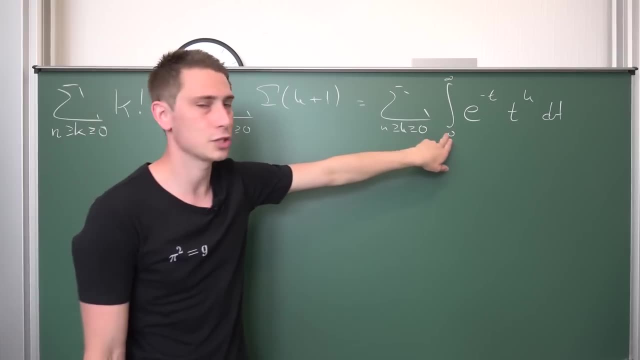 like this. it's going to be quite, quite nice now. at this point we are just having a finite sum here, meaning we can, without any further explanations, use the linearity of the integral to just interchange integral and final summation. here we are going to do this also. e to the negative, t is independent. 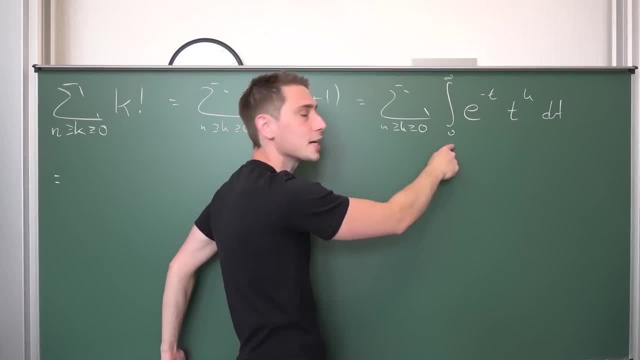 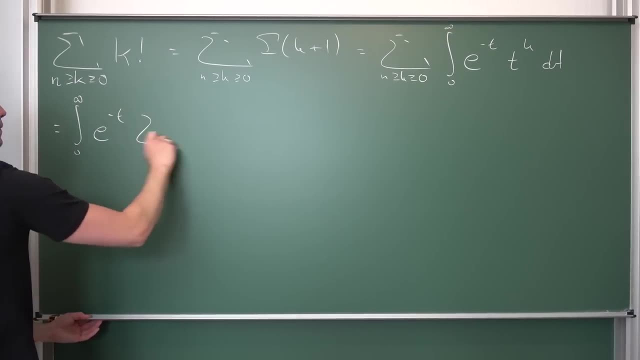 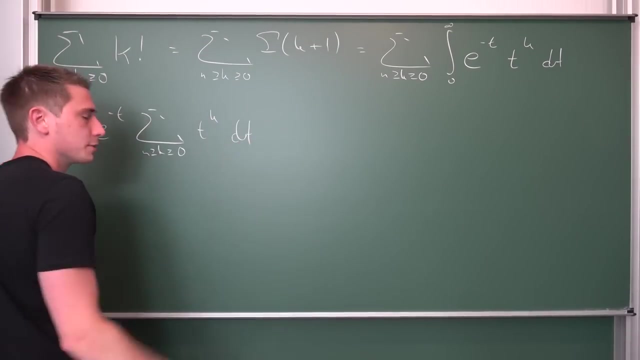 of the running index k. so let us bring it between the integral sign and our summation, leaving us with an integral from zero to infinity, of e to the negative t, finite t boy, where k is bounded between zero and n, of t to the kth power integrated with respect to t, and here's an absolute blessing. 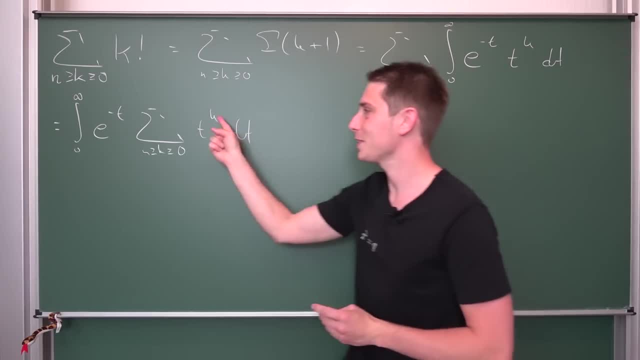 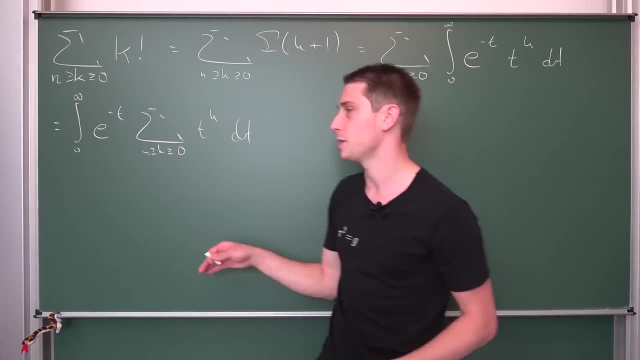 of god. this is a really good thing. this thing right here is just a geometric progression. i have derived it before. take the limit as n approaches infinity. we are going to talk about this in a second and you would have the geometric series not going to do this. this is just a simple. 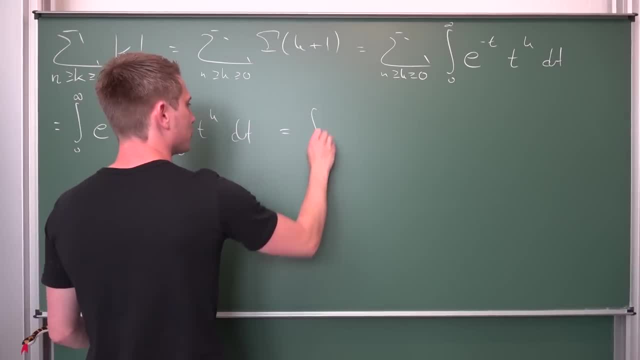 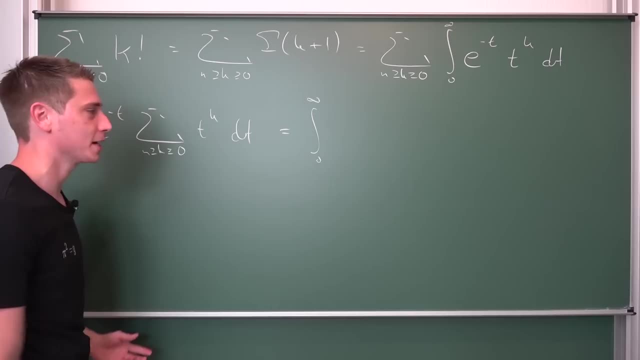 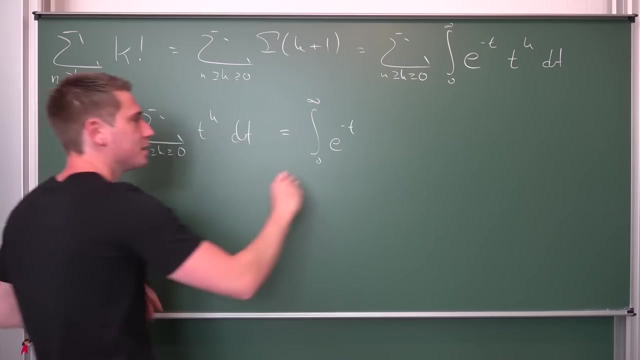 geometric progression, leaving us with integral after zero. oh, that's a sexy integral sign. oh, i'm so good at drawing these. that's the only thing i'm i'm really good at, to be honest. e to the negative t and the geometric progression gives us. so our upper bound for the summation is n. so t to the n, plus one power, minus one over t. 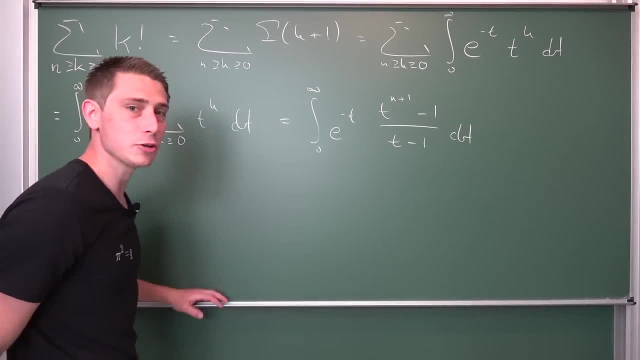 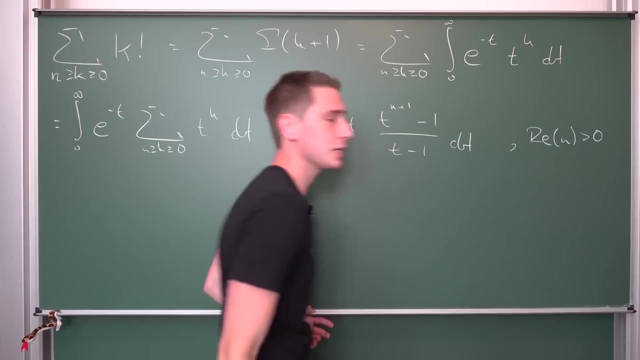 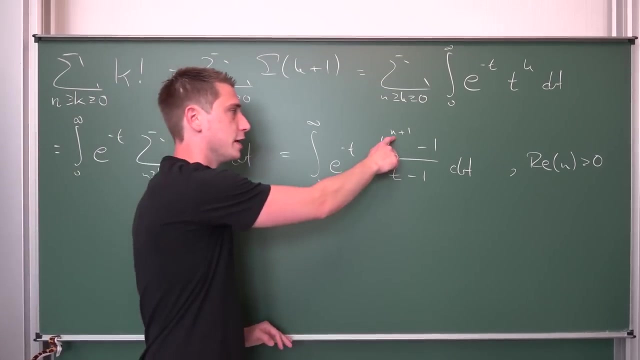 minus one, integrated with respect to t, and that's it already. this is an analytic continuation to the real part of n being greater than zero, and it's pretty amazing, right? i mean it looks fantastic. that's a really nice integral, and if you plug in integer values for n- positive integer values- then well, that works. 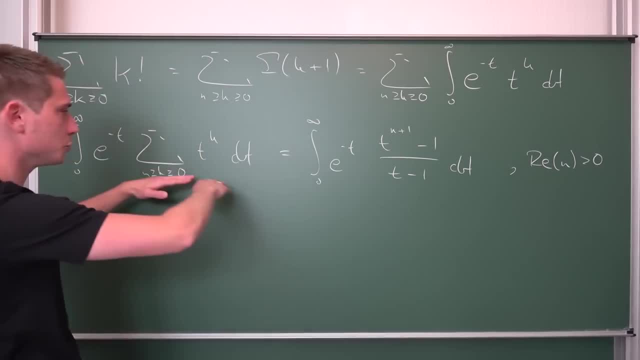 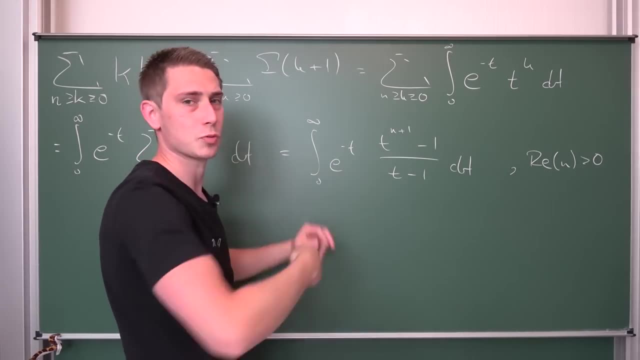 out quite nicely, because then our geometric progression is just going to reduce to what we have here. you can do integration by parts over and over again. n times it should be, or n minus one times. so it should be n times i. i think, yes, n times, and then you are going to end up with 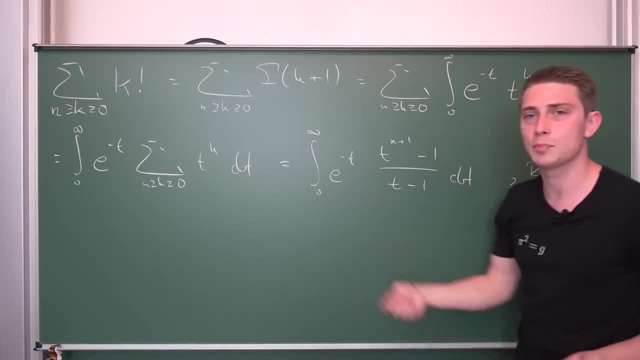 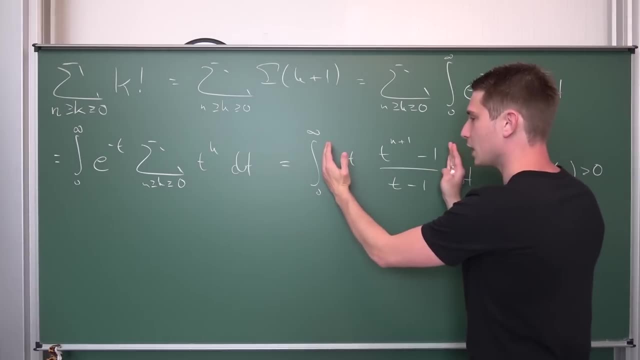 just the summation of t, and then you are going to end up with just the summation of t, and then we are going to end up with just this graphic definition up here. basically, it's a pretty nice thing, and we are now going to take a look at the graph of this infinite, because it's it's kind. 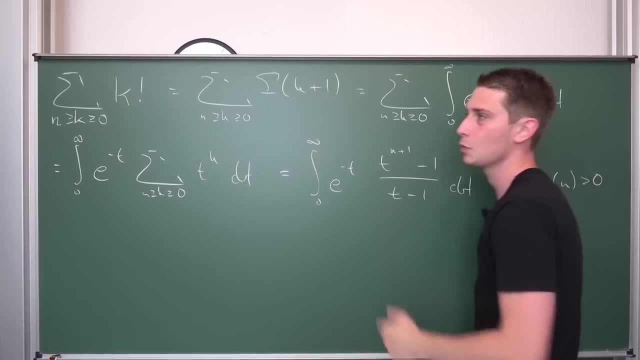 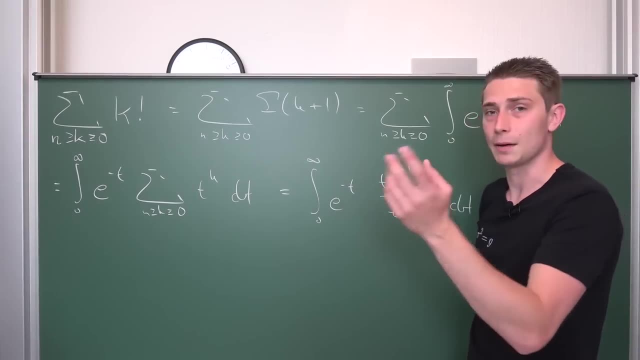 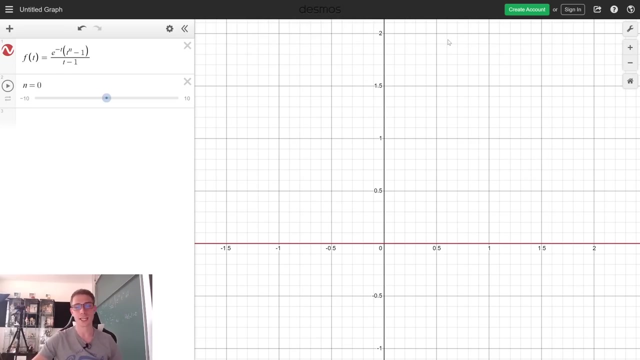 of interesting to look at what you are going to get out of here. even for for half values of n, for example, if you want to find a summation from one half 2 to 0 of k factorial, that that's also a thing. and yeah, here's the graph. all right, pulling off a little sag star, here we are going to take a. 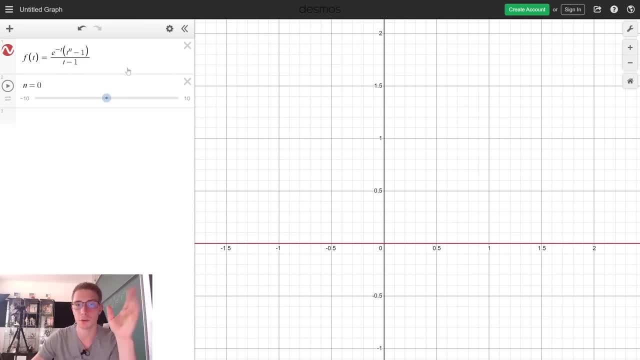 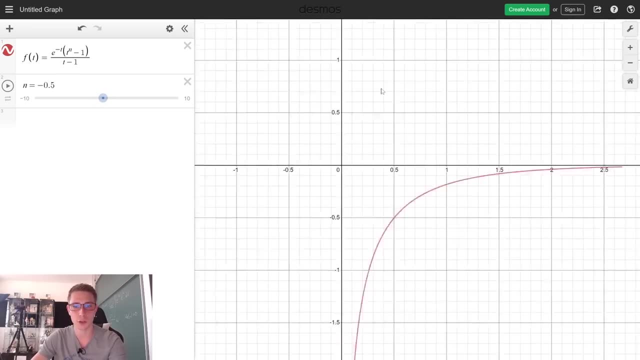 Or this representation is only defined for the real part of n being greater than zero. So I have put the integrand here and if we go into negative Territory then this whole thing is going to diverge. It won't work out. So this integral won't. 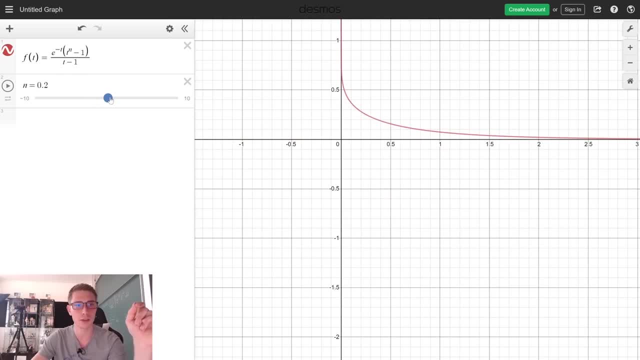 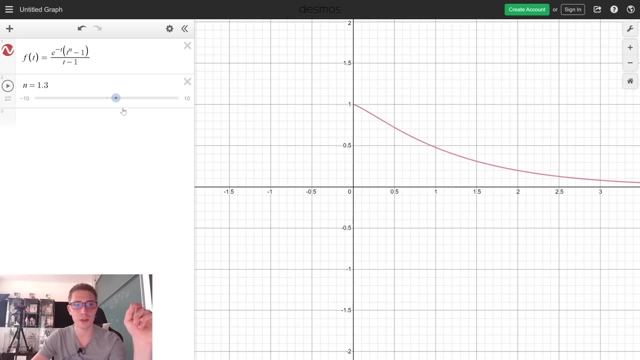 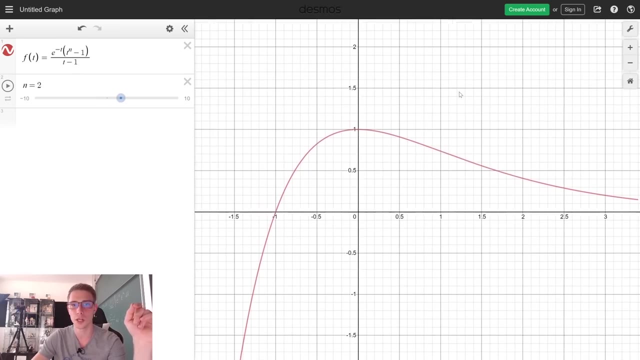 Exist for negative values, but if we take a look at positive values, You might notice that our graph is going to grow in some way. okay, if everything is between zero and Two, then the graph is still pretty nice to deal with. so the curve looks nice and sleek. 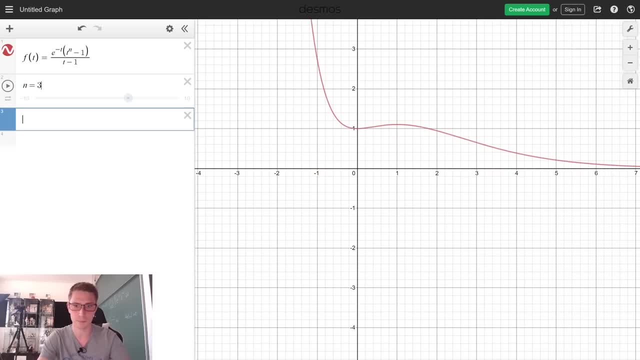 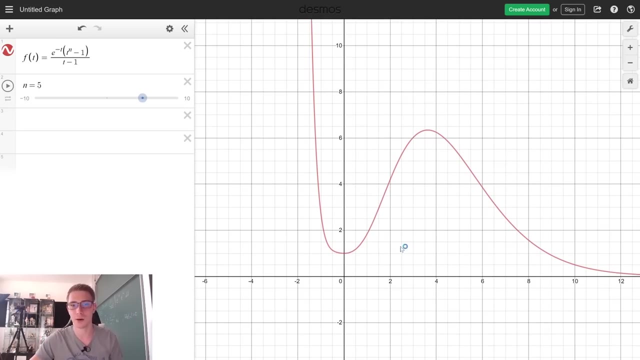 But once we start going higher, for example three, Well, there we go, Curve is growing. What about four, Oh goodness. What about five, Oh damn. Look at that. now, at five it already starts exploding. But this comes in quite natural because, you see, our integral is just: 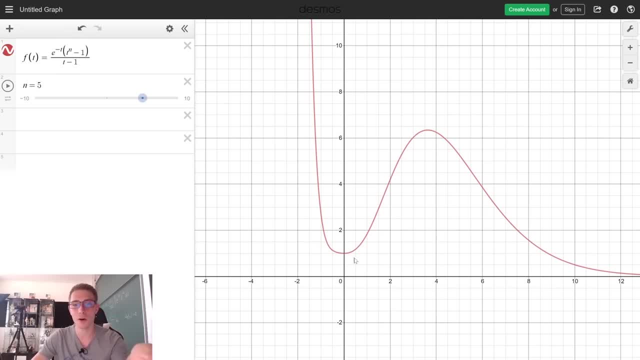 The area are under this curve, meaning overall that our 5 factorial as the upper bound is going to be 5 factorial plus 4 factorial plus 3 factorial plus 2. blah, blah, blah, And 5 factorial is already a lot of stuff. It's already. let me think for a second. 1 times, 2 times, 3 times 4 is going to give us. 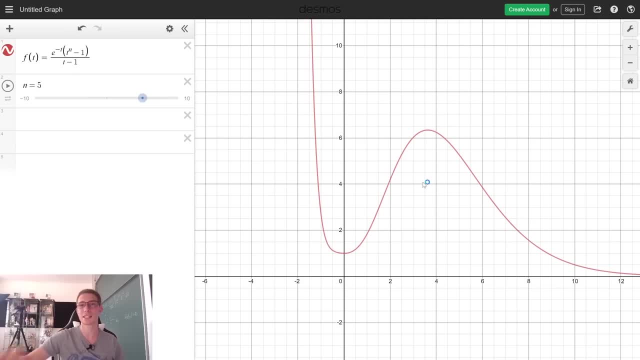 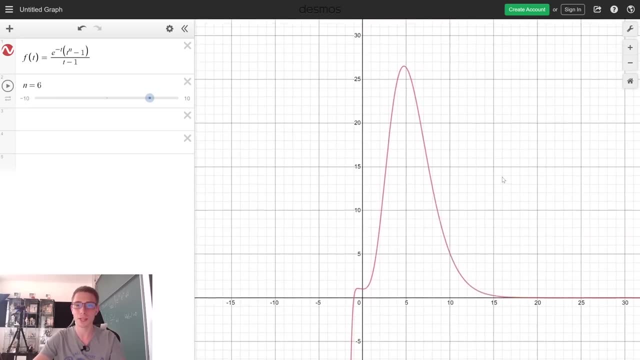 24,, ah, 120 already. And if you add this stuff up it's just going to grow so damn hard. So let's take a look at, oh goodness, 6.. It's exploding so hard. Now let us zoom out really hard. and now for number 7.. 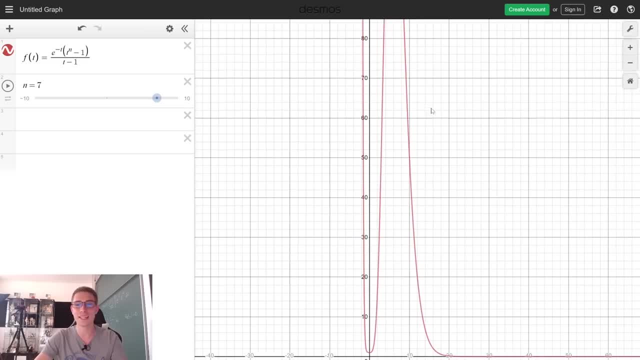 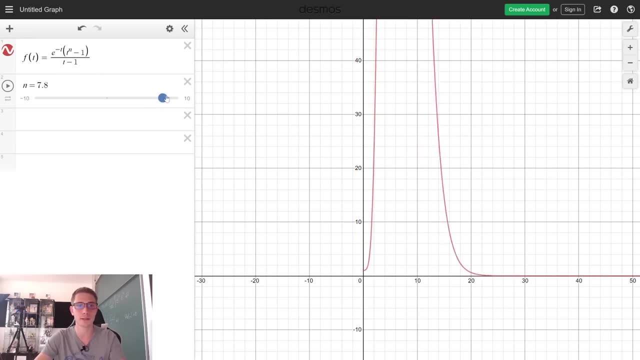 I can't even fit it on the screen already. You see, the area under this curve is just going to explode, and here's a nice and basic, intuitive understanding about this. It's just going to diverge for really big values of n, This integral, for n approaching infinity, is just going to diverge, which does make perfect. 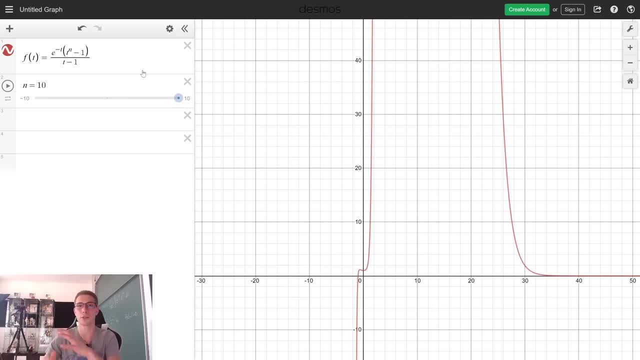 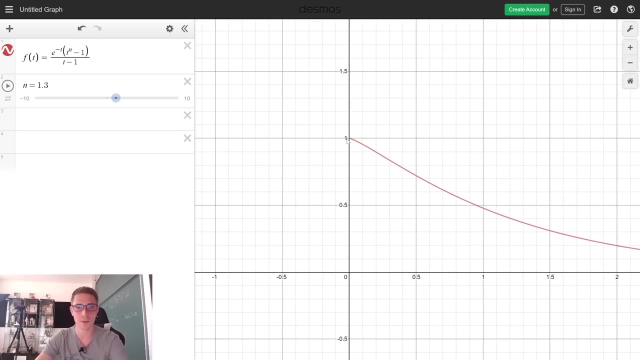 sense because, well, we are adding up positive stuff. We just get so much bigger over time. Factorious grows so extremely hard. And other than that, one cool thing I would like to take a look at is if we zoom in yet again, if we take a look at: yeah, this is a really nice curve, just stopping at the 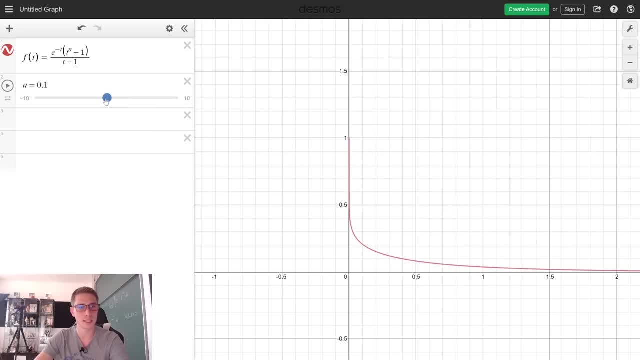 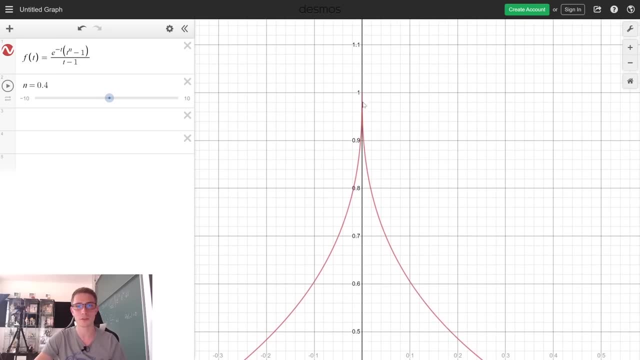 number 1 there. But if we just take a look at 0.4, this is quite an interesting thing. 0.4 looks like it's not continuously differentiable here, So it's not differentiable in 1, which is kind of curious. 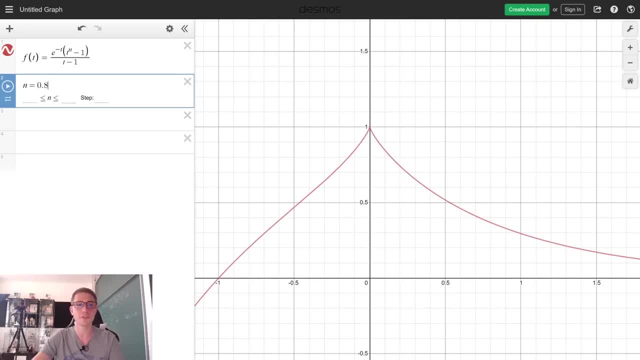 Then if we go up to 0.8, we have the same situation In 0.4 steps up until 2.0, it's going to look quite weird. 1.2, you see, now it's getting kind of smooth here. 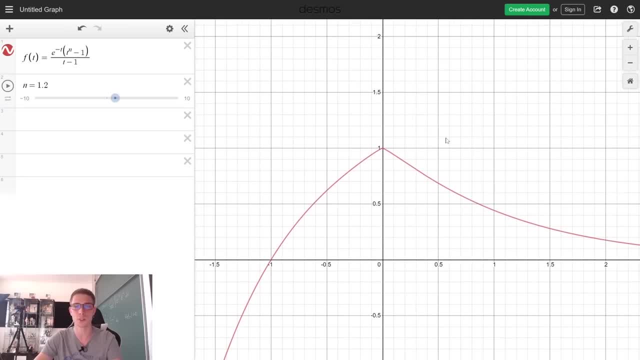 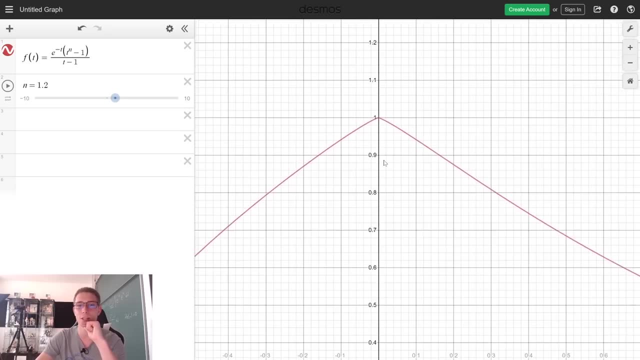 I'm not certain if it's differentiable there for like values between 0 and 1, where it's a multiple of 0.4.. So 0.4 and 0.8.. I'm not certain about the differentiability there. 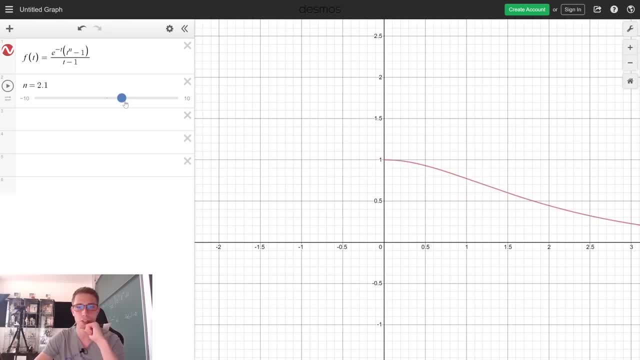 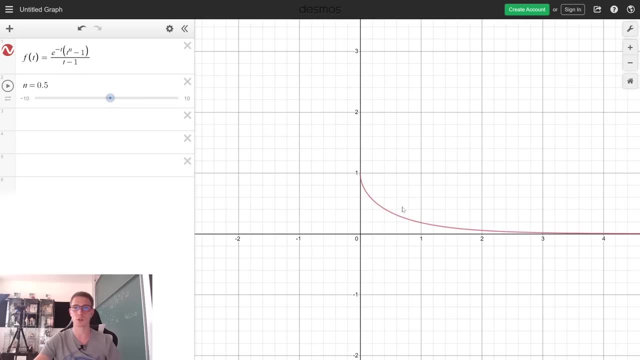 This is just a nice little observation I have noticed, Yeah, Other than that really cool stuff here. If we put 1.5 here, for example, then the area under this curve is going to represent like the sum of factorials up until 1.5 factorial, whatever this is supposed to mean. all right, 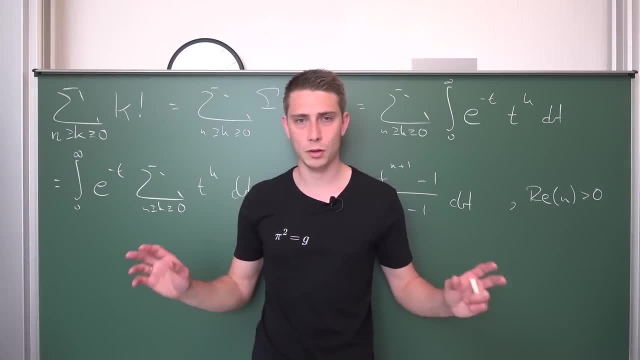 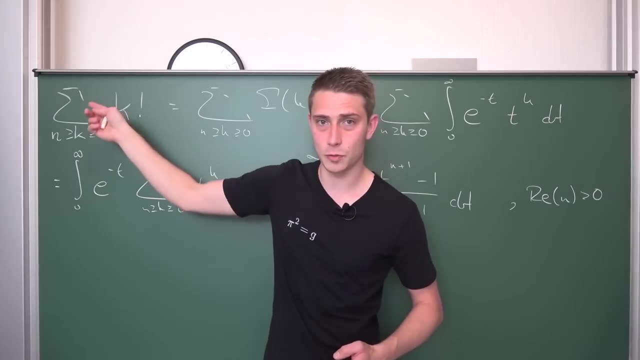 I hope this little insight was to your liking. Back to the blackboard. And now here's a little bit more background information and the functional equation for this thing actually is a really cool thing. That's a function with respect to n. okay. 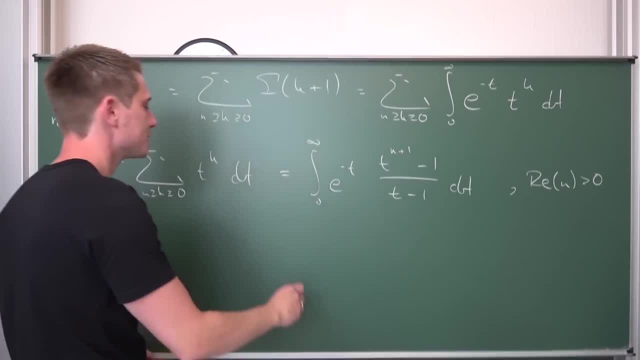 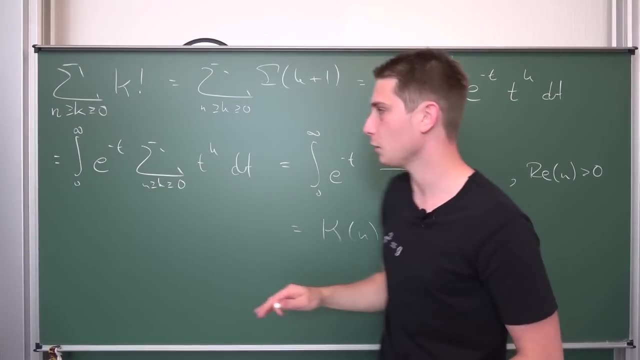 It's dependent on the variable n, And this thing is actually called curretas Sum of currepa's function k of n, And it's a well-known thing. I have derived it for myself, though, So I derived this integral representation for myself. 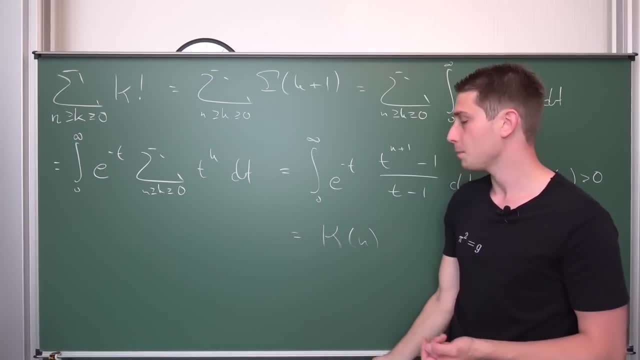 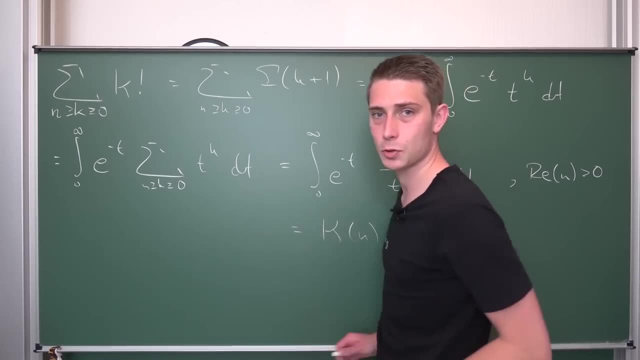 It's not really hard. You see, it's like a two-liner, It's not too much work. But it's still kind of interesting that someone has dealt with this before And currepa has found another expression for this thing involving exponential integrals. 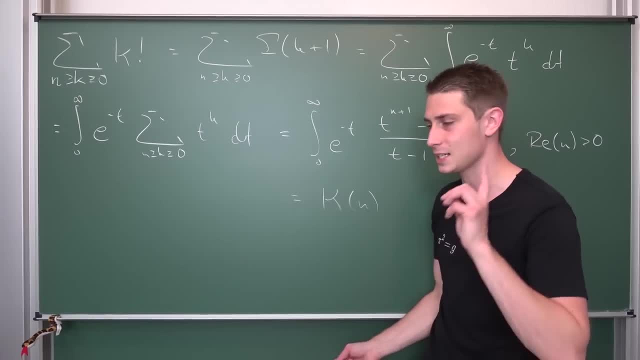 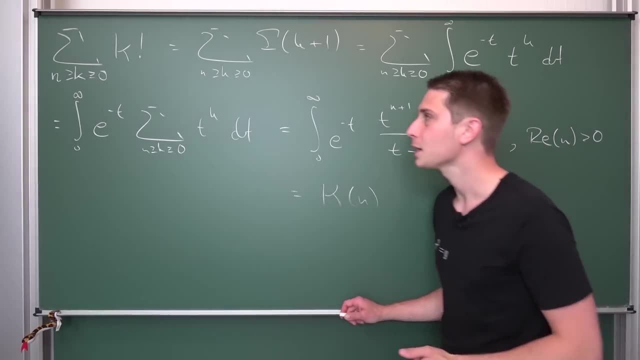 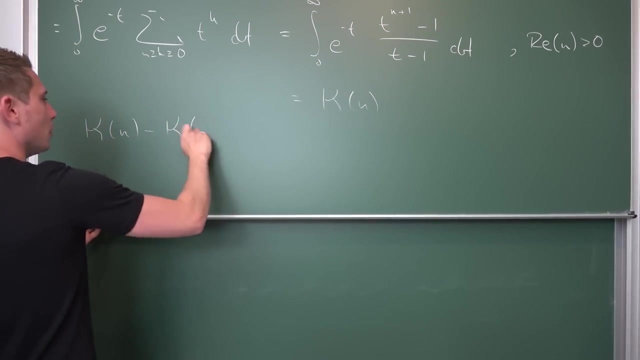 It's an absolute monster. So deriving this is really not easy. It's really Not trivial. Other than that, there's a cool functional equation for this thing. You might notice that if we take the difference of currepa of n and currepa of n minus 1, what? 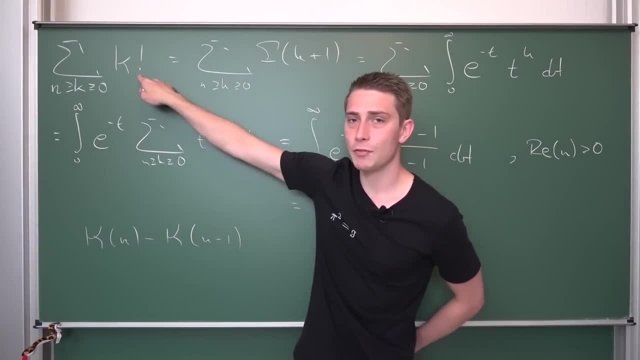 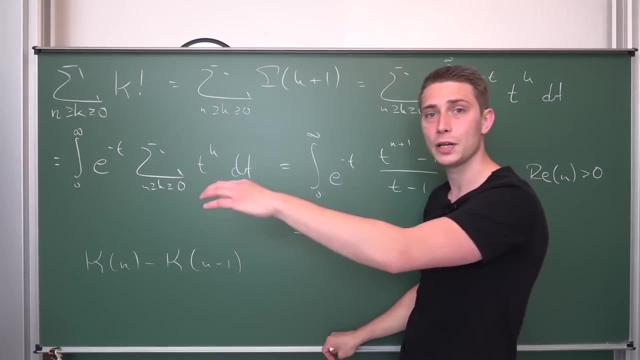 is it going to relate to. So currepa of n is nothing but n factorial plus n minus 1 factorial plus blah blah blah, up until 0 factorial. And currepa of n minus 1 is n minus 1 factorial plus n minus 2 factorial up until 0 factorial. 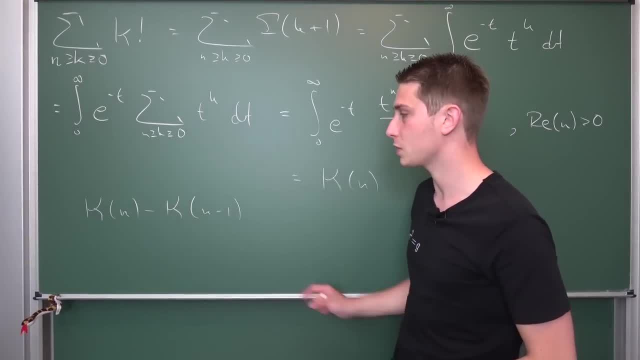 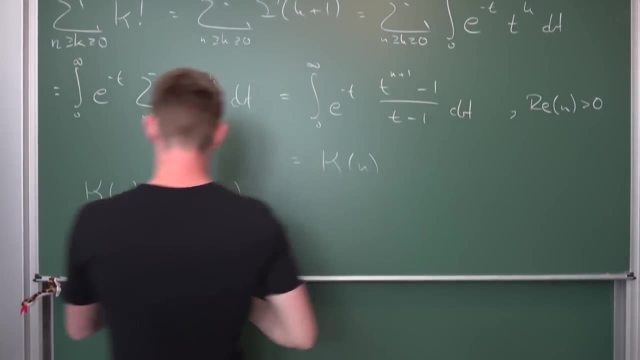 And all the parts Starting from n minus 1 factorial are going to cancel out in the summation, leaving us just with n factorial at the end And n factorial. okay, I'm going to write this out: this is n. factorial is nothing. 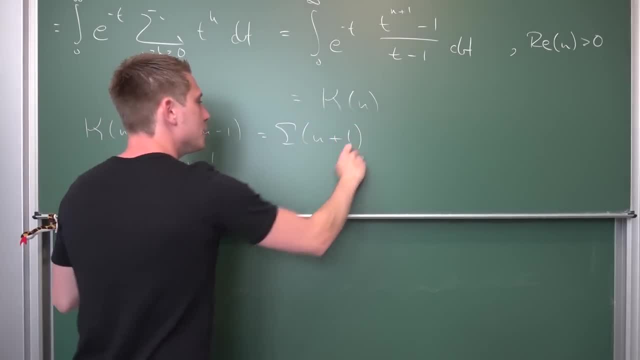 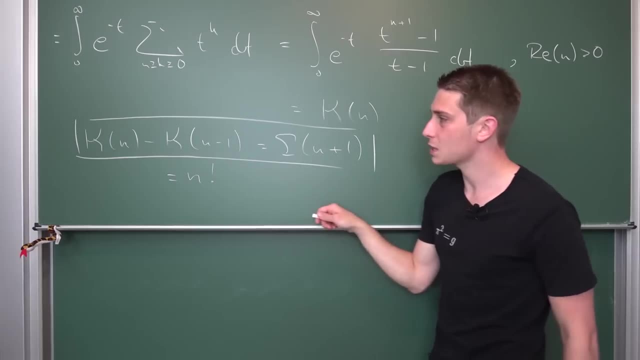 but well, gamma of n plus 1.. So the really cool thing about this is that there's a really nice functional equation here which looks kind of like the functional equation for the digamma functions, for example, or the trigamma functions or polygamma functions. 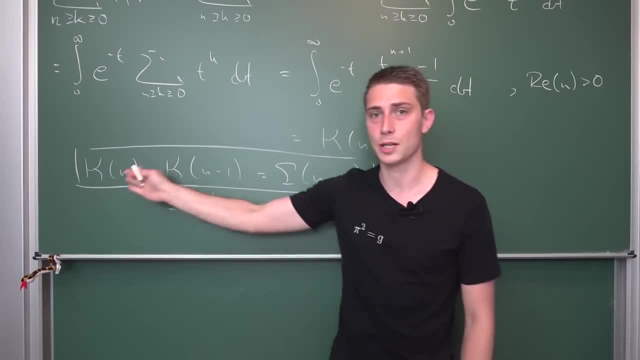 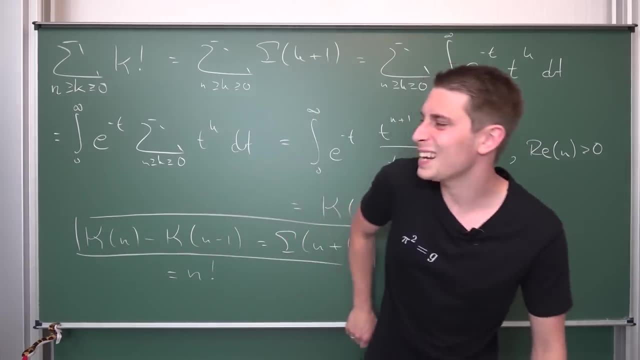 It's pretty interesting, if you ask me. So that's a really nice connection between the gamma function and currepa's function. If you have any further questions, please leave them down in the comments below. And other than that, I would like to thank Brian for sponsoring this episode of some. 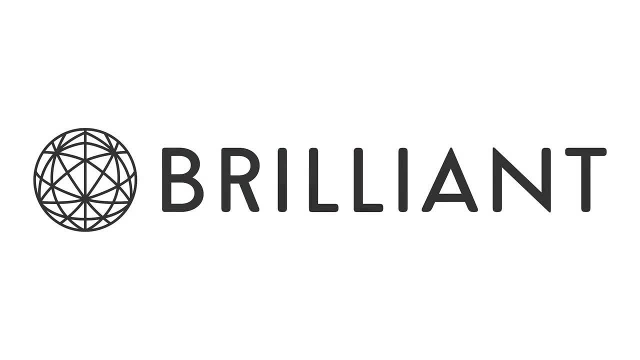 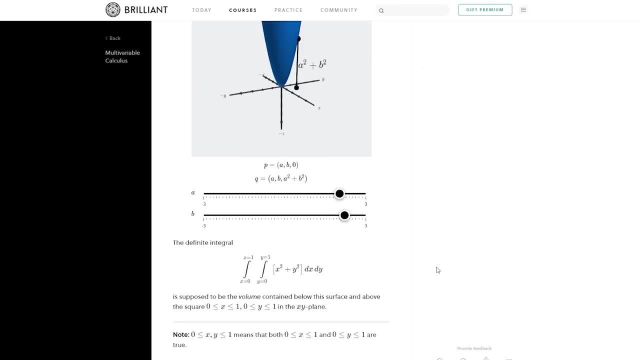 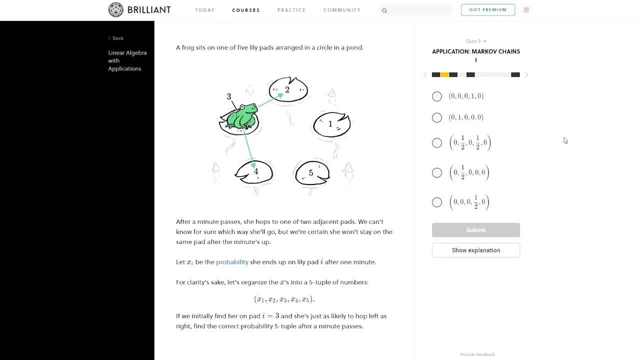 more analytic number theory here. I hope you enjoyed this analytic number theory goodie featuring a rarely occurring special function. I really enjoy working through such intimidating looking problems that turn out to yield such sleek solutions. If you also find joy in playing around with integrals, summations, and like to simply 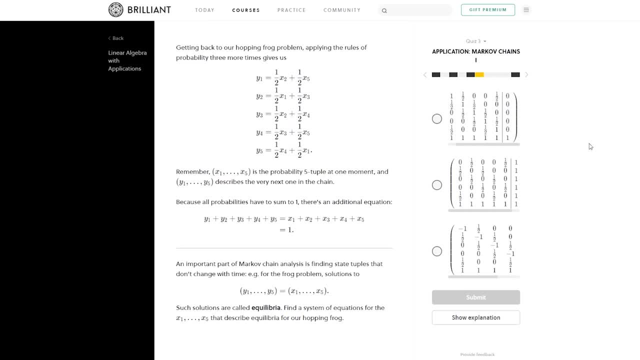 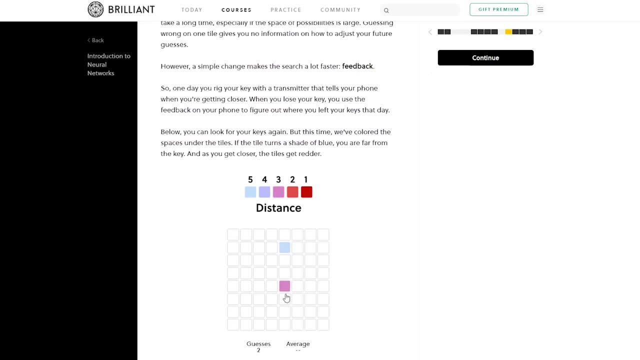 try out new and exciting mathematical tricks, then Braiant could be the perfect fit for you. Braiant is an online learning platform and app which focuses on active learning and problem solving. Braiant can help you achieve your STEM goals by working through their over 60 interactive 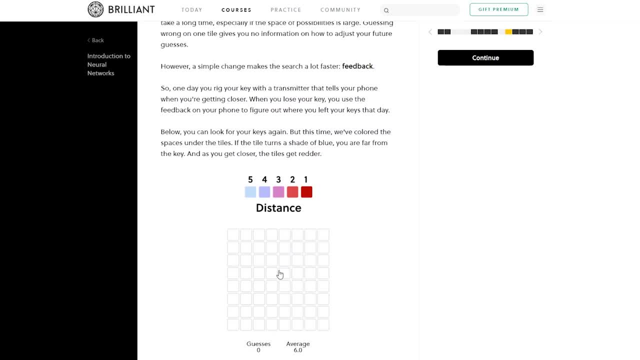 courses in maths, computer science and all sorts of scientific disciplines. A huge variety of mathematics-oriented content. to play around with. Braiant is a platform for you. to play around with. Braiant can help you achieve your STEM goals by working through their over 60 interactive 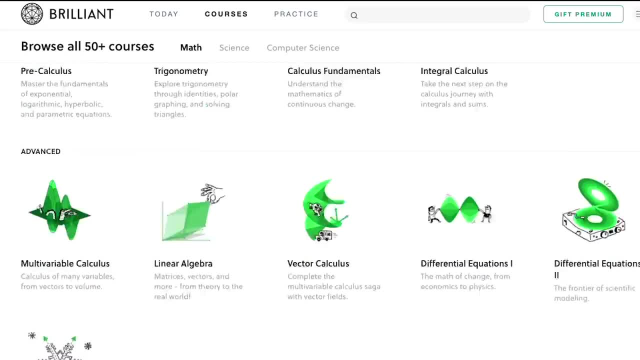 courses in maths, computer science and all sorts of scientific disciplines. You can find them on many of their Parents there and hopefully, if you are a kid, there can be a time for this. We have adequately slopes in purpose and we injured the. 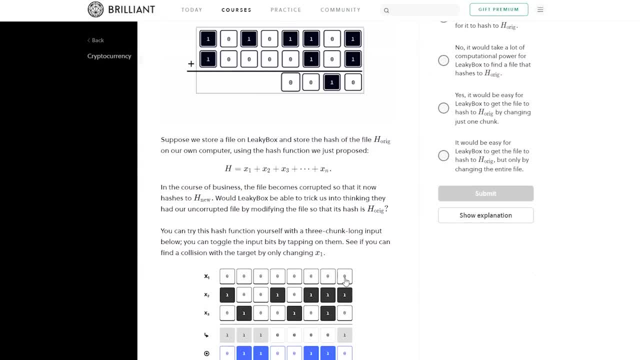 loans to make sure we don't have anymore apps there Now. this is an extremely important piece, so if you are a parent of a child or a teen, whether it's children's and mother's day, we are very happy to share it with you. 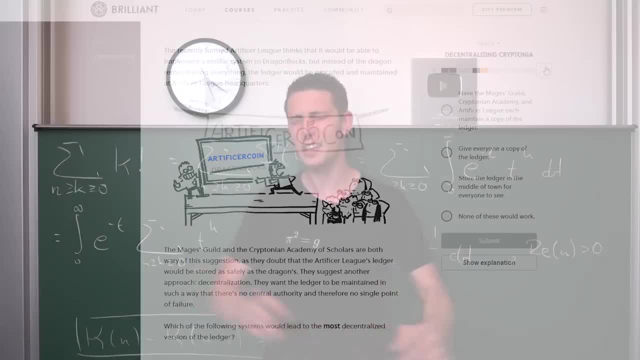 It will help you achieve these goals. Once again, thanks for making theimbussioncom an option for design and sorry if my English is not very fluent, but it will both help this video work and make it work천ushiro治 team more successfully. 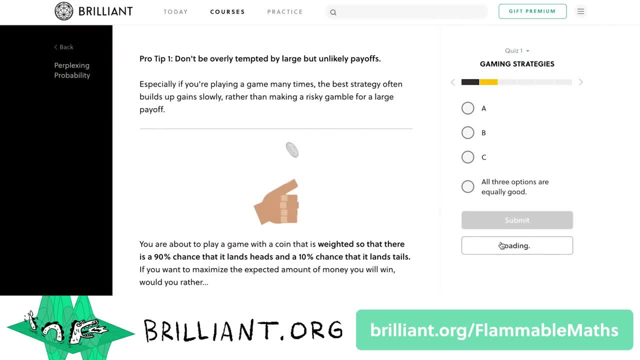 omas обрат wants to thank you very much because the amount of story and understanding You can get completely free access to brilliant and, the first time, the people to actually completely use the link at 20% of an annual premium subscription, which is a really good. 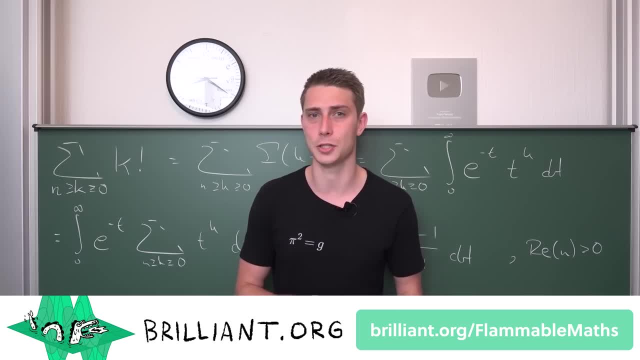 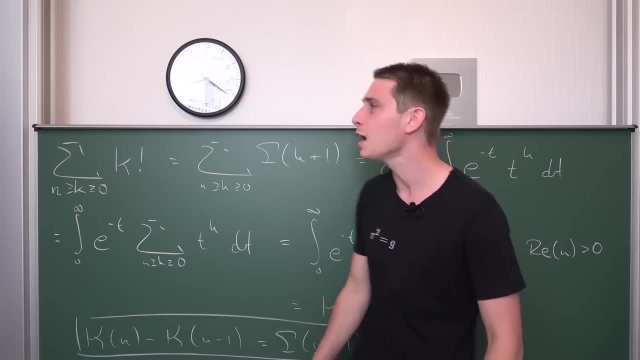 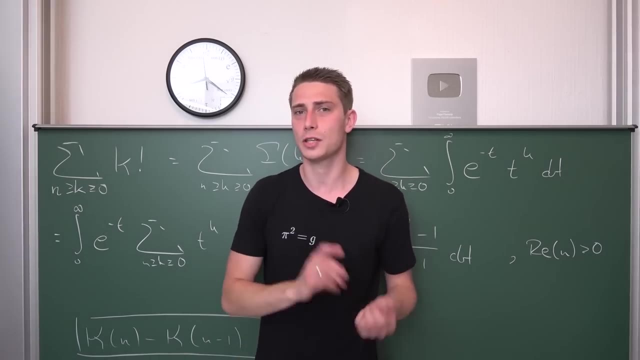 deal, considering how much content they have on their website up until this point. So try it out and support the channel this way, and I thank you guys for watching. If you didn't join this video, please subscribe. recommend channel flag. Also, engineering war clock only available for one and a half months, 200 pieces, limited.